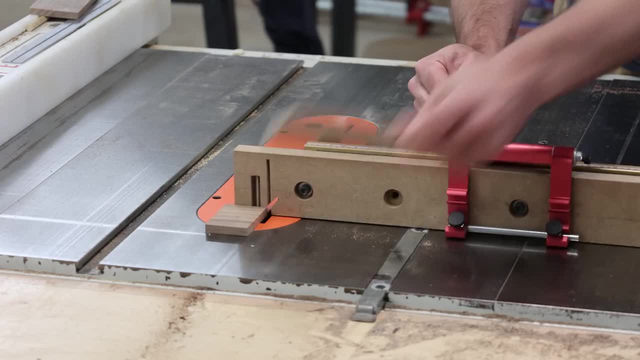 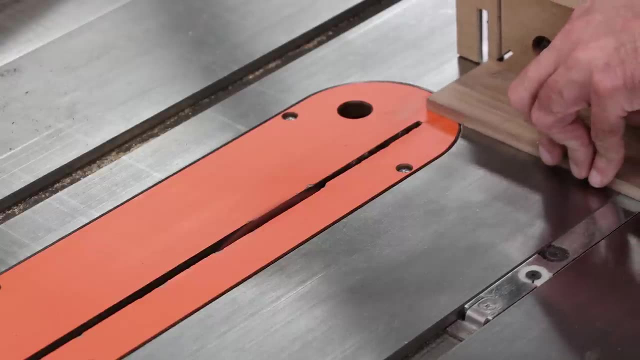 that's what my eyeball said looks really good. I do most of my work at the table saw, So I cut my long and short pieces using the miter gauge, but you could also use a miter saw too. When it comes to joinery, I recommend keeping it simple. If you decide you want to go with crazy dovetails, 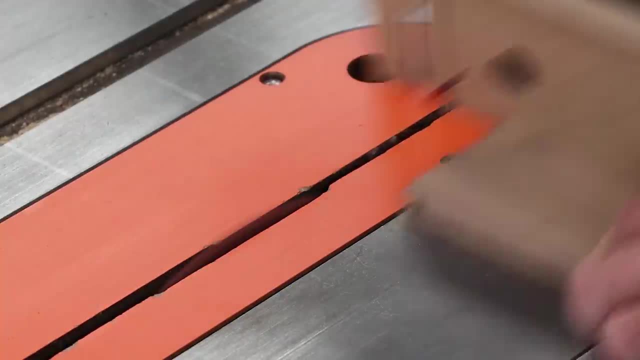 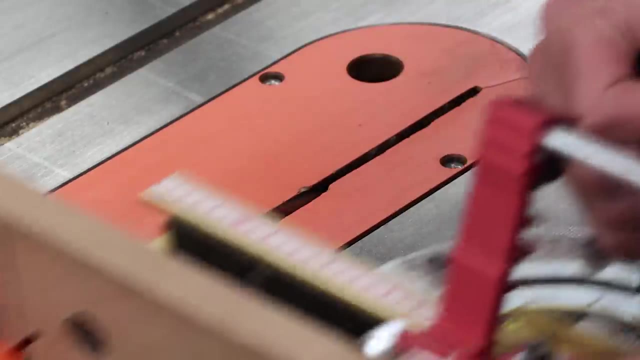 well, that's going to be added labor, which means your price is probably going to go up. So for my little box here I decided to use rabbet joints. I lowered the blade down to about half the thickness of my workpiece and then nibbled away the underside of my two long pieces until the 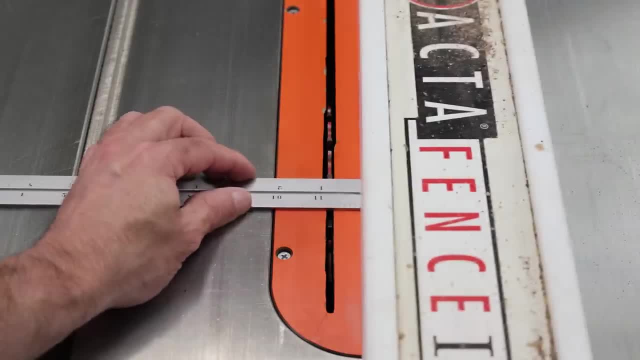 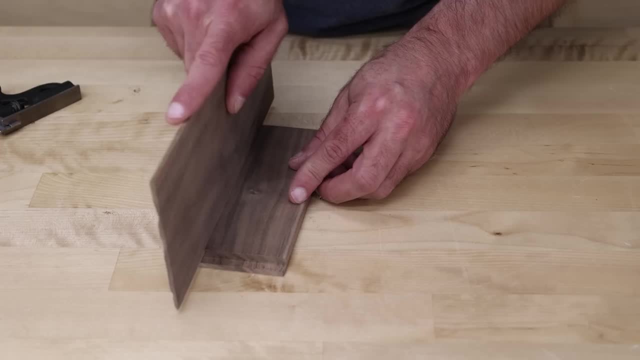 short side fit flush into the long side. My box bottom is going to be a quarter inch thick board. Using the table saw I cut a groove on the inside face of all four of my pieces. bump the fence over just a little bit made another pass. 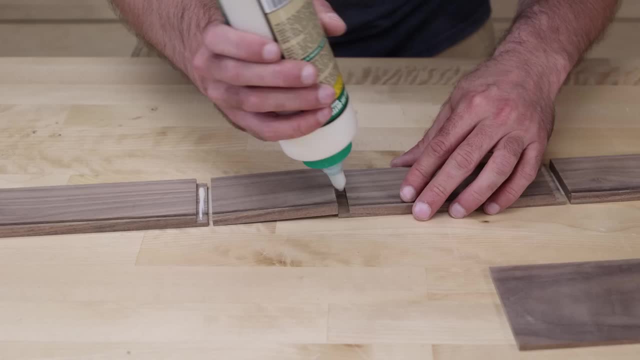 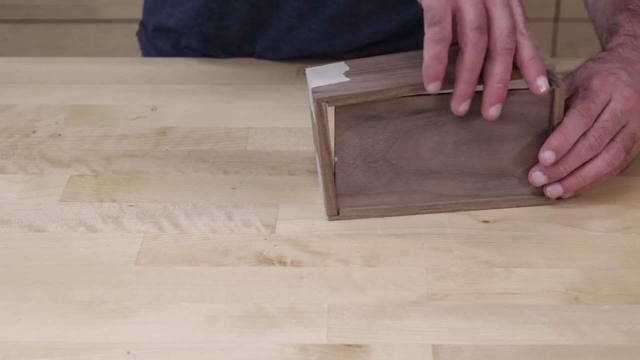 until that board fit nicely into that groove. If you're making a lot of these at one time, that means you're going to use a lot of clamps, or you can do what I do, which is use masking tape or painter's tape. Make sure you squeeze all those joints really tight, tape it with a whole bunch of. 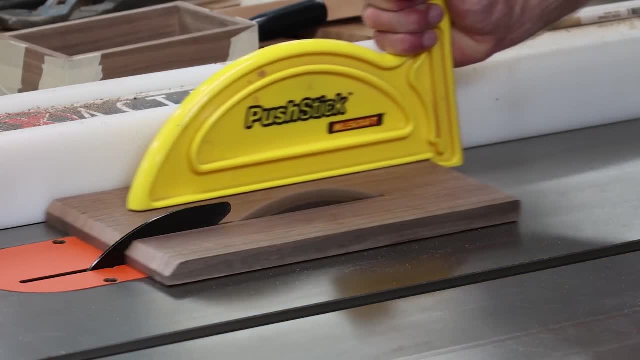 tape. let it dry. While the glue's drying, we can start working on the lid. I like to have my lids be removable, because hinges add extra strength to the wood, So I'm going to use a little bit of extra tape to make sure it fits perfectly. I'm going to use a little bit of tape to make sure it. 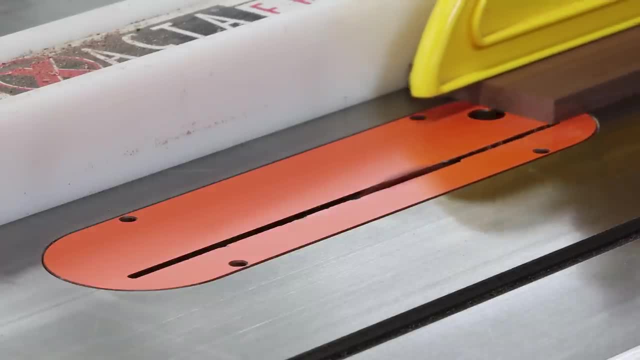 fits perfectly. I'm going to go ahead and trim the edge of the board so I can add extra work to it. I'm going to cut the side of the board to about an inch thick and then I cut it to its final size, making sure that it's about a quarter inch extra on all four sides of the actual box itself. I want. 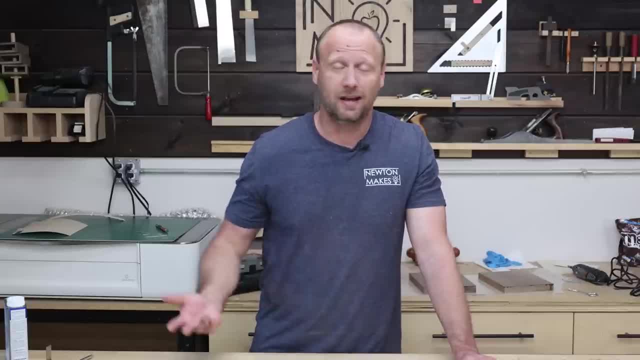 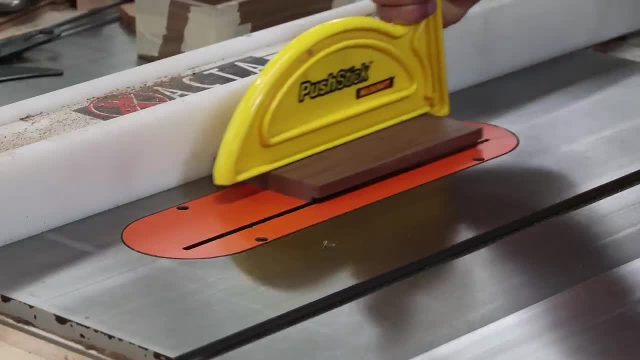 to have a little bit of overhang there. Now, this quarter inch measurement I completely made up, so feel free to make up your own measurements. I lowered the saw blade down to about 1⁄8 of an inch tall, maybe a little higher. I'm just making it up And then I cut the long sides. I make a. 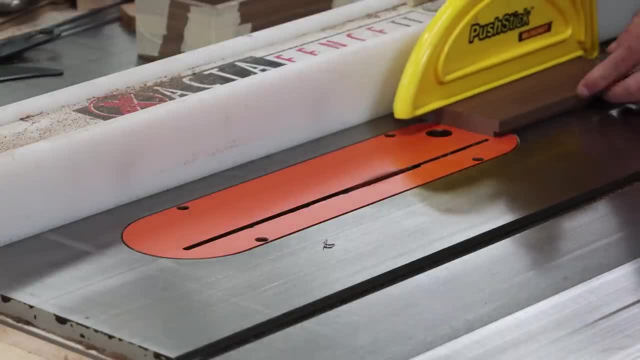 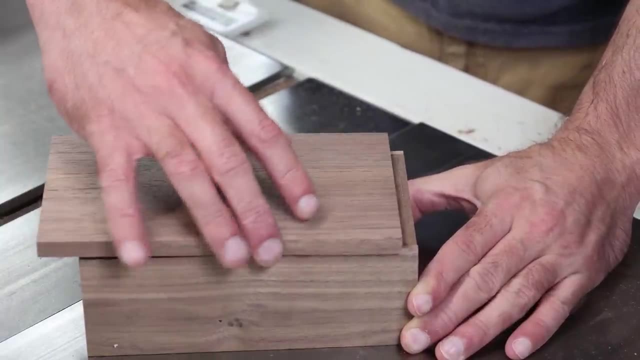 pass. I rotate the board around and then I cut the other side, Bump the fence over a little bit. it do the same thing: cut one side, rotate it around, cut the other side, and i'll keep doing that until the box lid fits into the box. i do the same thing for the short sides, i just use a miter gauge. 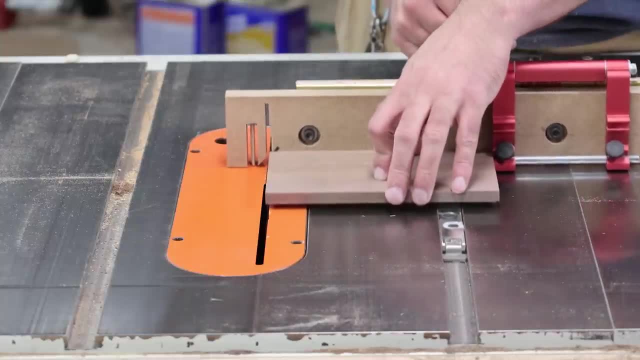 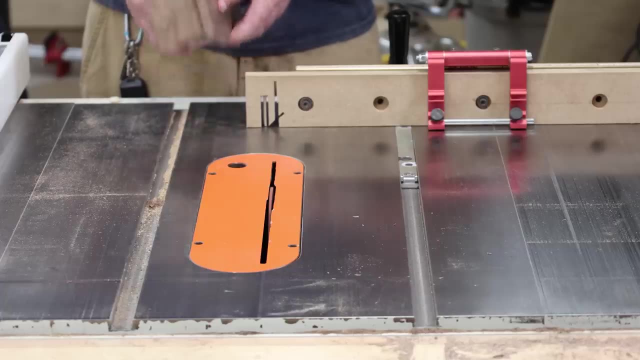 instead of using the fence. but i'll make a pass. rotate the board around, make a pass. move my stop lock over. make a pass. rotate it around, make a pass until the lid fits into the box the way it's supposed to be. a little sanding and we have us a beautiful looking box. now these things sell. 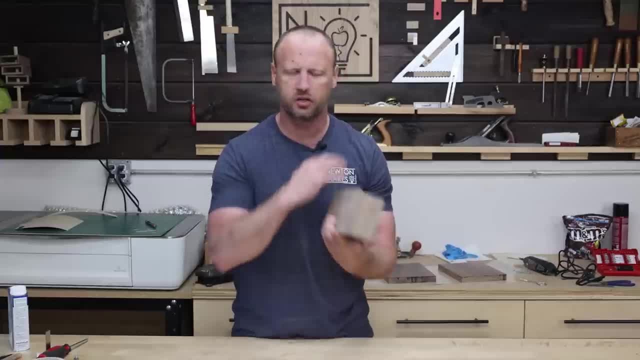 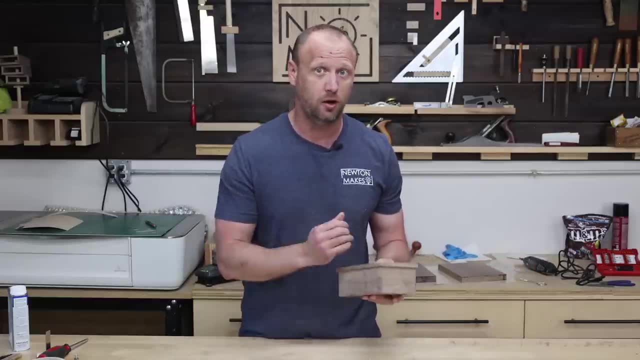 really quick, especially if you do any sort of personalization, engraving cnc, whatever on them. now, this took me maybe an hour or so to make. but don't just make one, because you need to maximize your profits, which means make a bunch of them, batch them out, five, ten at one time. you're going. 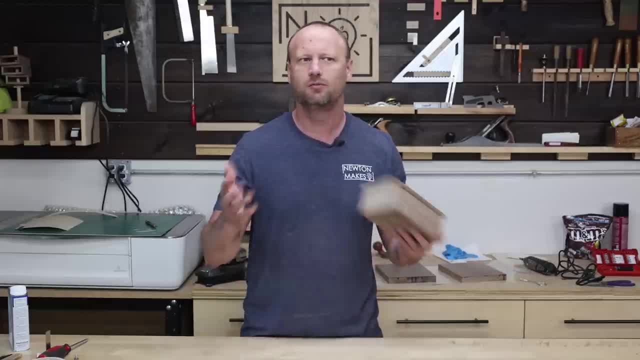 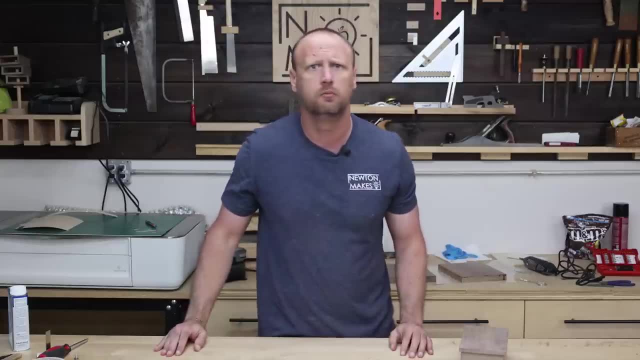 to sell them. so that's going to help you out that way and also it's just way easier. you set up your tools one time you make a cut, you just keep batching all the way through. so now that we got this done, uh, what's next? okay, this next project's. 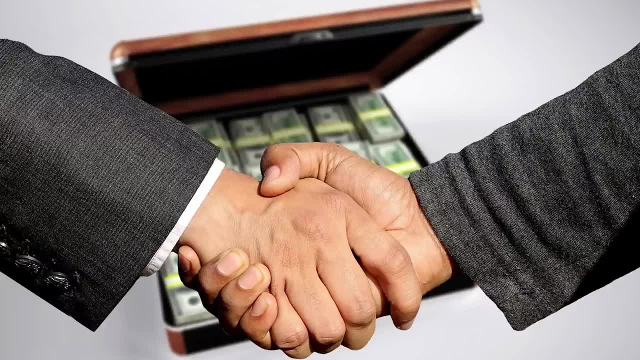 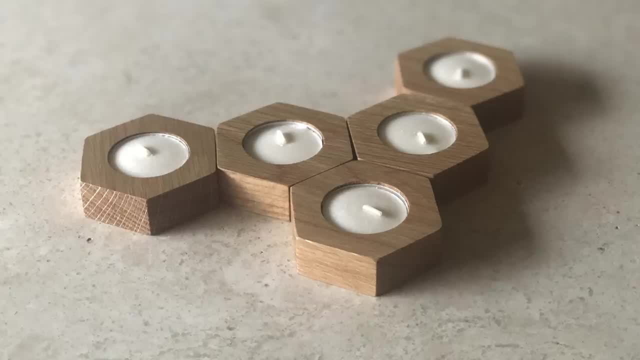 going to seem almost too simple, and i thought the same thing until i started selling them like crazy, which are tea light candle holders. i would make hexagon shaped candle holders and sell them as sets, and they would sell out quite often. there are multiple ways to cut hexagons. now one way: you. 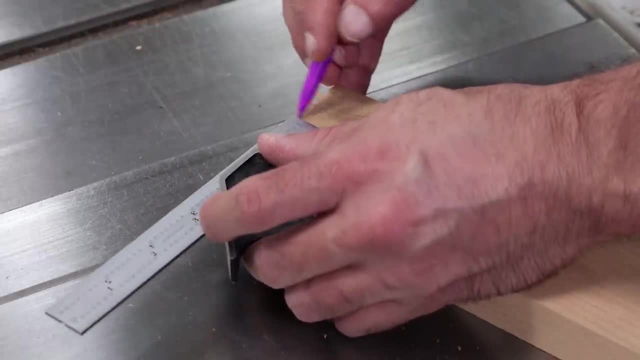 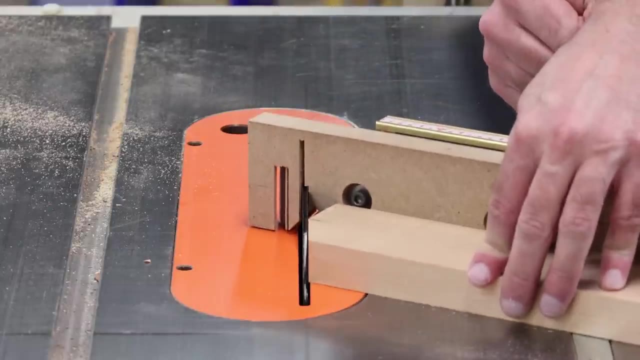 can do. it is using the table saw. so i will mark the center point of my board, then i'll turn my miter gauge to 30 degrees and then i'll make cuts sneaking up on it until i hit that center point, flip the board over and then cut the other side. 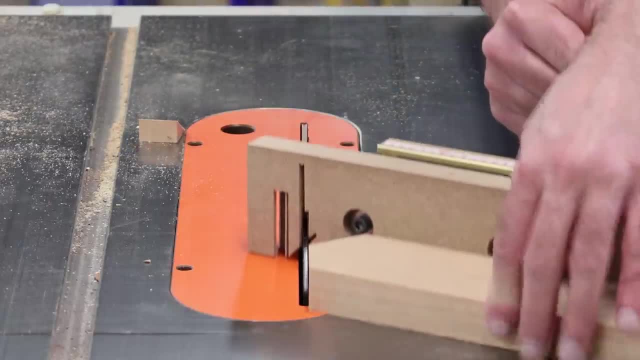 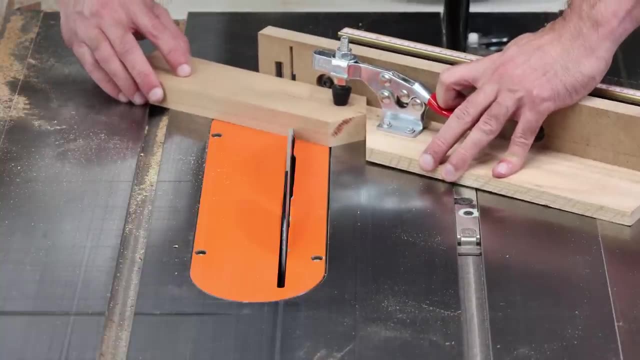 that takes care of one side of your hexagon. i cut the scrap board to 30 degrees and this is just a quick little jig to help hold the candle holder in place. now i also added a toggle clamp onto that to help hold the board in place, so i don't have to put my hands close to the blade and then i don't. 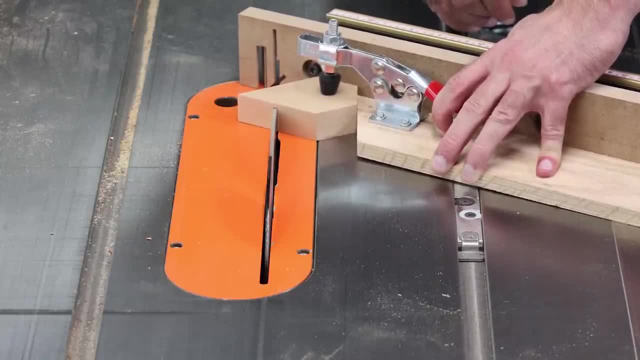 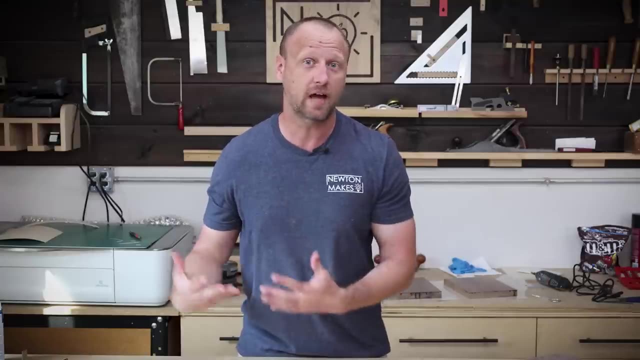 accidentally, you know, cut my body in half, cut one side, flip the board over, cut the other side. now you got a hexagon. this is something that you're going to want to make efficiently and be able to batch out, so you need to come up with a way to make them quick and safely. 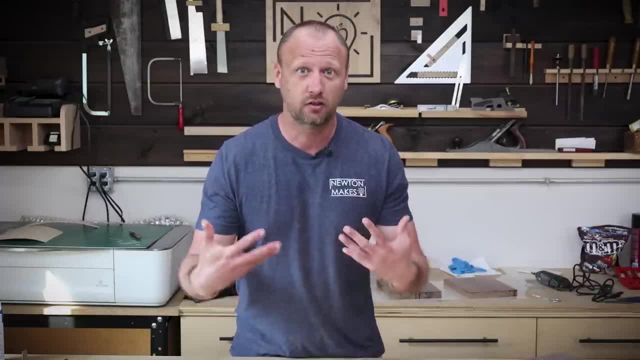 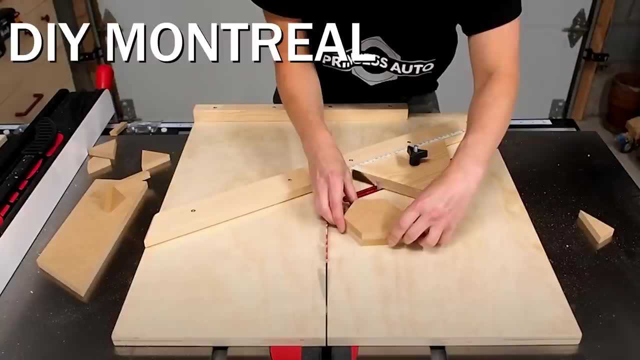 and all repeatable, so i would recommend making a dedicated jig to this, based off the size of the candle holders you want to make the diy. montreal has a fantastic video on how she made a sled to do this, so i would definitely check out that video, because that sled she came up with is 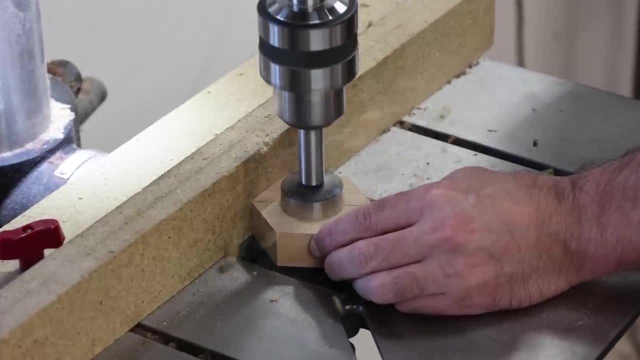 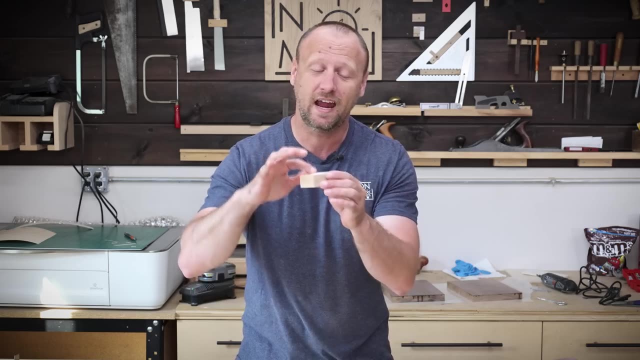 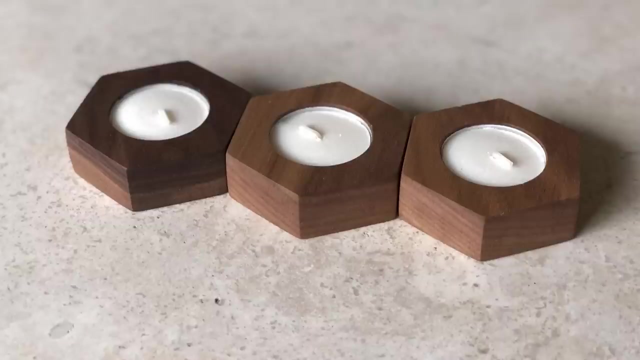 absolutely perfect. mark the center point of your hexagon and, using a one and a half inch diameter forster bit, drill a hole about a half inch deep. this is the perfect size hole to hold a little bit of wood to keep the lizards in place, and then, if you do need some extra help with that, you also. 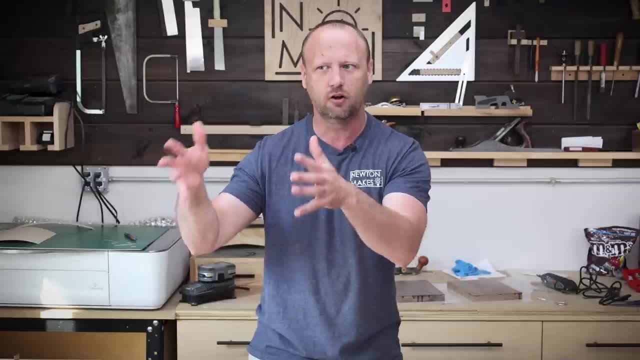 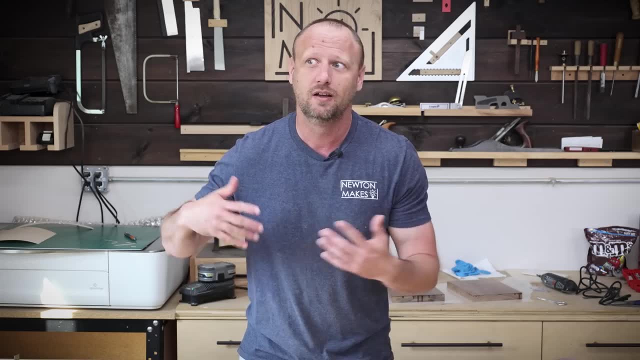 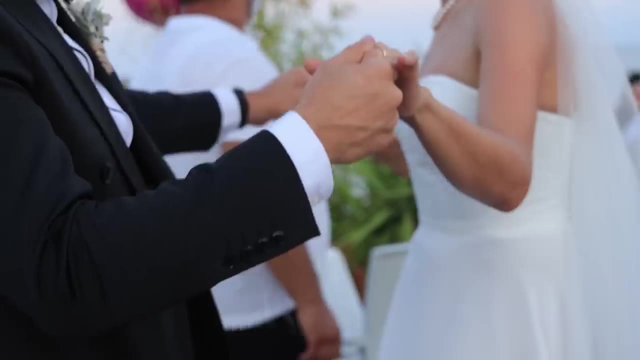 want to build a little big wood to hold it in place. i'm not going to spoil it much, because i would love to build something big out of your wood. that way, when people are looking at your listing online, they will see they get the candle holders and all the candles all together and the candles are easily replaceable, because just about everyone 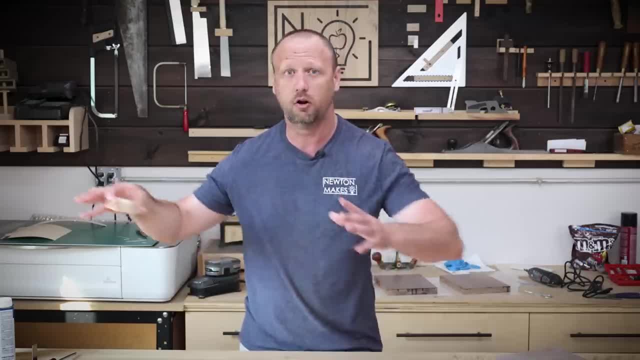 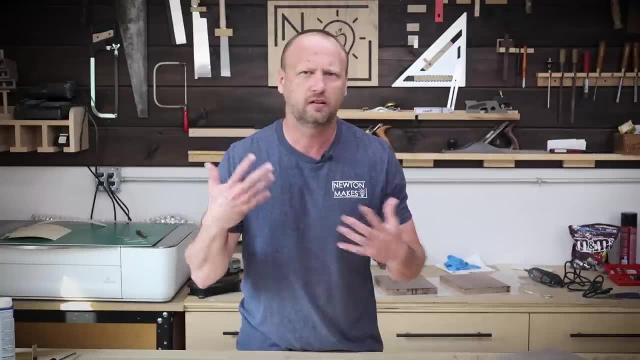 in the united states has a target nearby. you want to start really batching these things out in the for wedding receptions to put on the tables. Also, there's a lot of houses that are purchased in the summer months. People are always looking for that perfect housewarming gift. 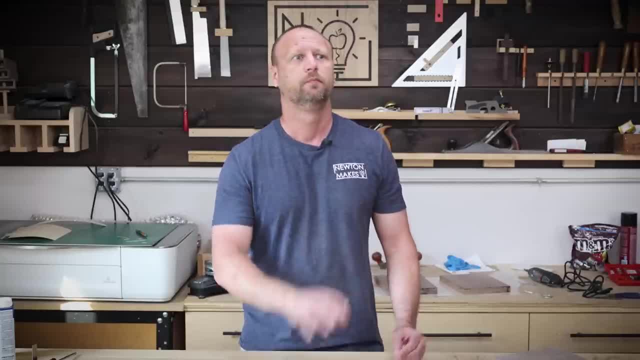 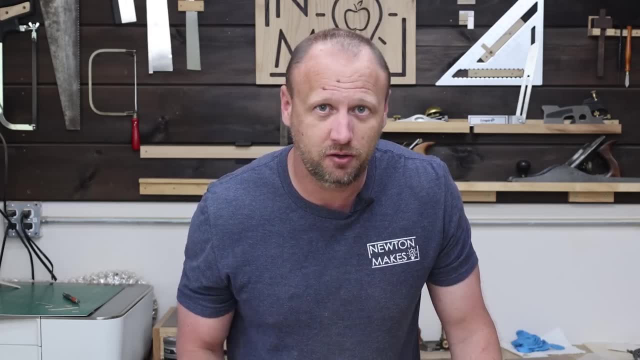 and well, these fit that bill. Another, Another. Before I get into the third video, let me give a big shout out to the members of our superhero community over on Patreon. Members like Brad Chaney really help out this channel and allow me to do what I do. 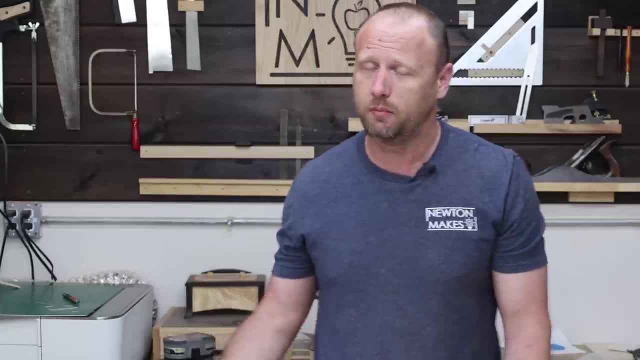 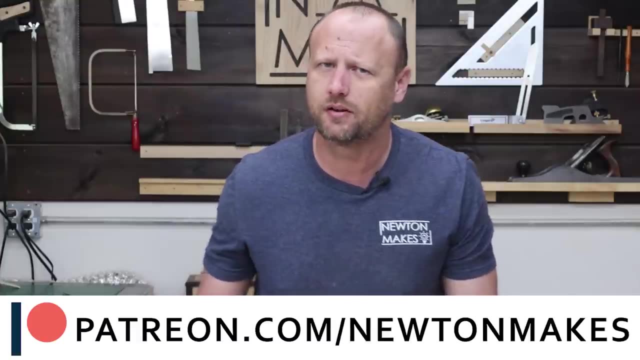 Members get extra footage behind the scenes- sneak peeks, woodworking plans- and their support goes a long way into helping this channel grow. So if you are interested, then head on over to patreoncom, slash newtonmakes and sign up Our third woodworking project that sells. 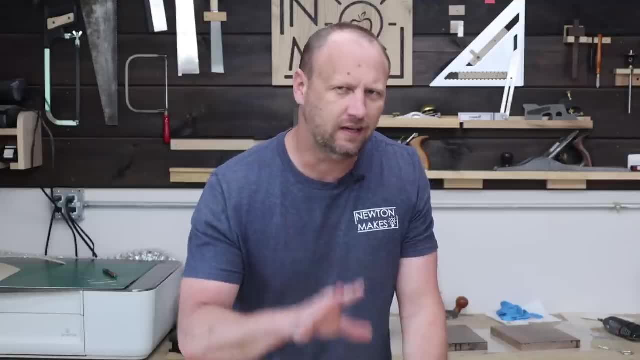 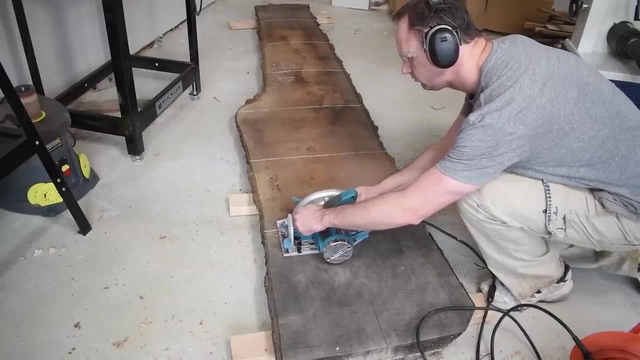 is any sort of unique serving boards Unique? that is the key to this. I like to let nature do all the talking with this. So anything that's live edge, that natural edge of logs or slabs, or you can even take some firewood and cut it up. 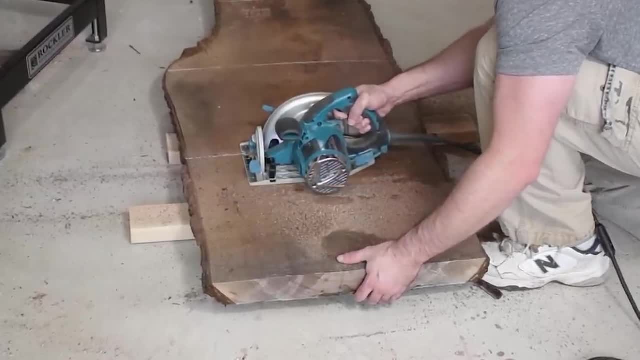 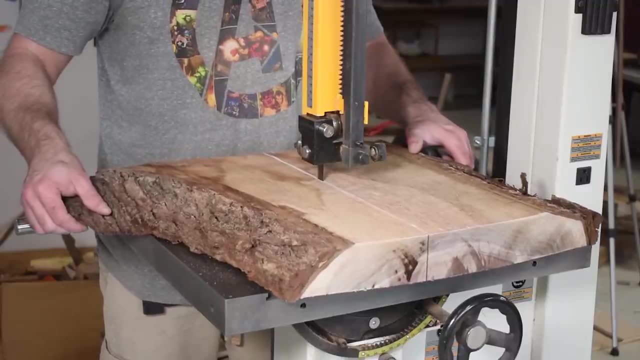 and make a serving board out of it, but keep that live edge on one side at least. those are big sellers, especially if you're dealing with dark woods, Your walnuts, your cherries, those are always gonna do better as a serving board. 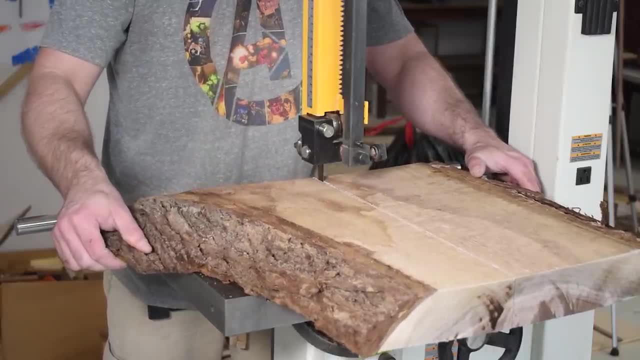 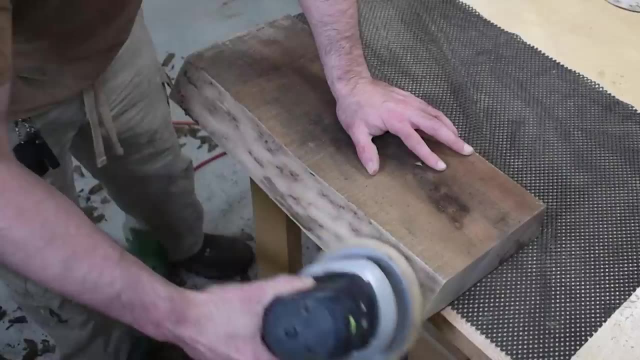 than something like maple. They're one of the easiest projects to batch out because they're kind of simple. if you really think about it, You're gonna do some sanding. You might plane it down a little bit just to get it nice and flat. 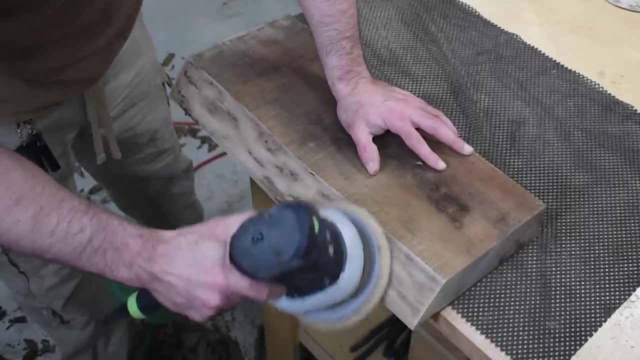 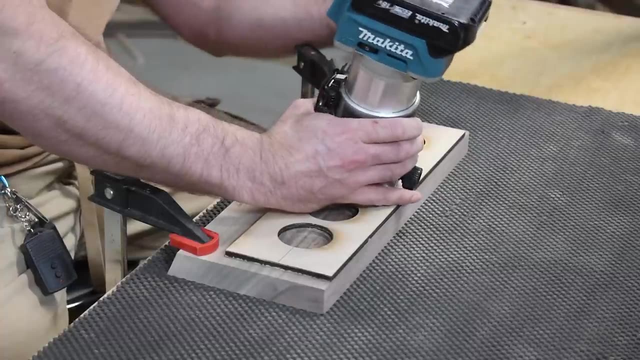 You might wanna put a bevel on the bottom, just so it's a little bit easier to pick up. but all in all, not really a whole lot going on here. You can make them for a specific purpose, such as a shot flight or a beer flight. 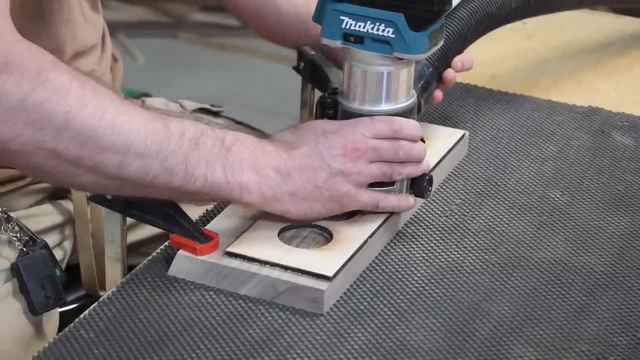 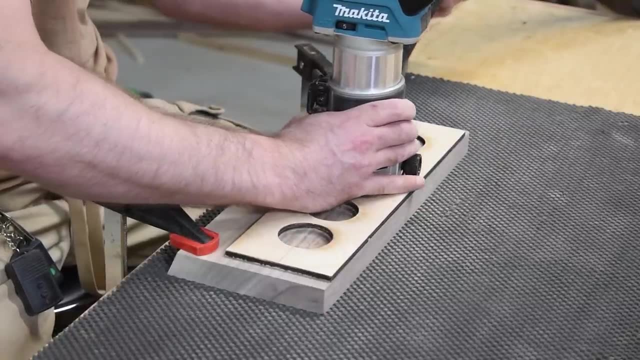 You know, take your router, ride out some circles in that thing or route out a big tray in it so that you can put food, snacks, whatever in it, So you can make them to serve you a specific purpose. but in my experience kind of done it both ways. 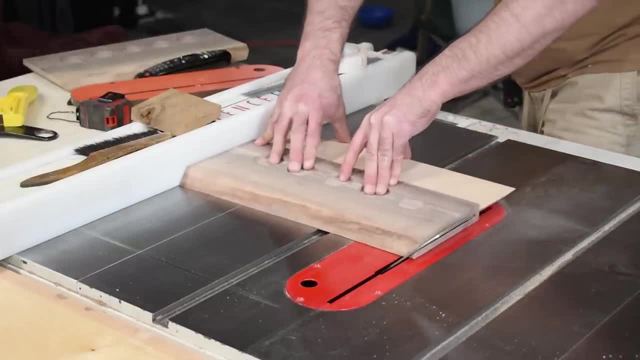 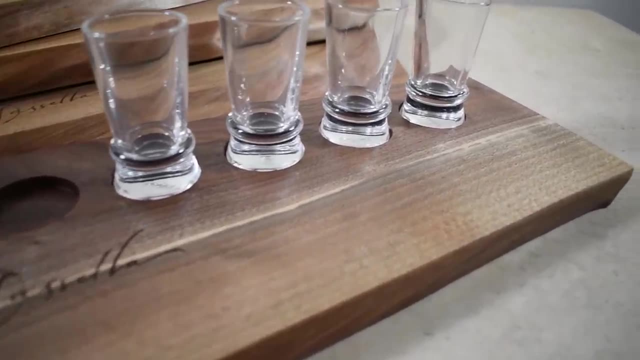 I've made a lot of them, especially for particular restaurants where they wanted a bunch of different flights. Also, I've sold a ton of them that are just plain, because they're universal and anybody could use them for whatever. I put live edge projects in a different category. 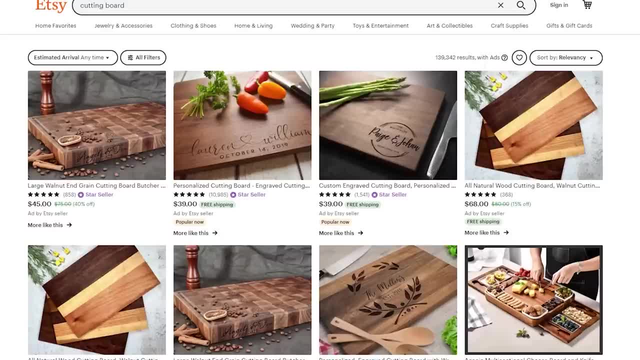 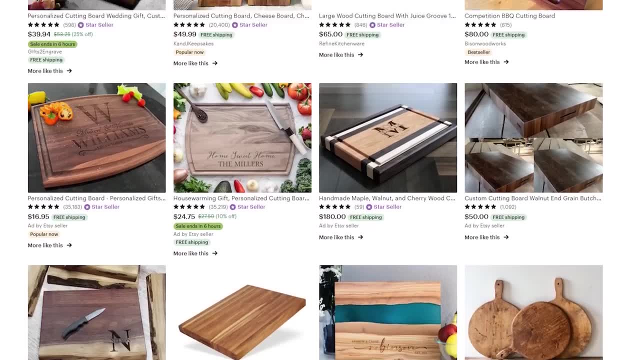 than I would. a typical cutting board because of the competition. Go on to Etsy and look up cutting boards And you'll see that all those top sellers sell a ton of cutting boards but at the same time they don't necessarily make them. 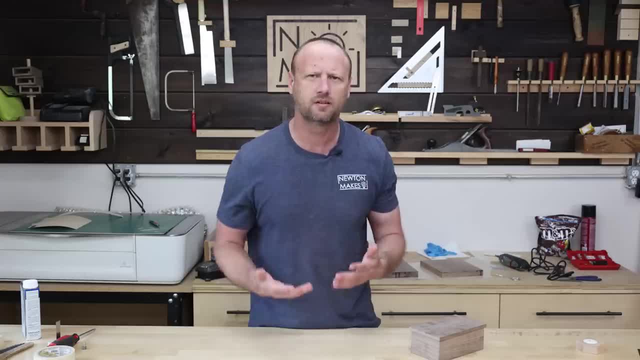 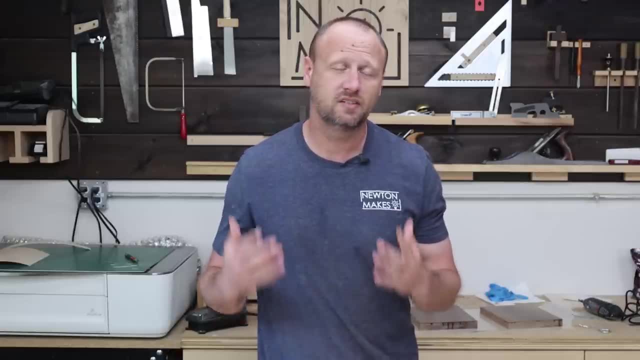 You can tell they buy them in bulk, probably for just a couple bucks each, And then all they really do is provide the engraving, which is their version of uniqueness. As a one man shop, I just can't compete with those sorts of prices. 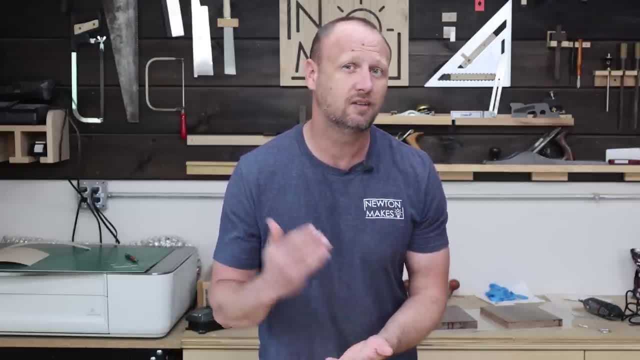 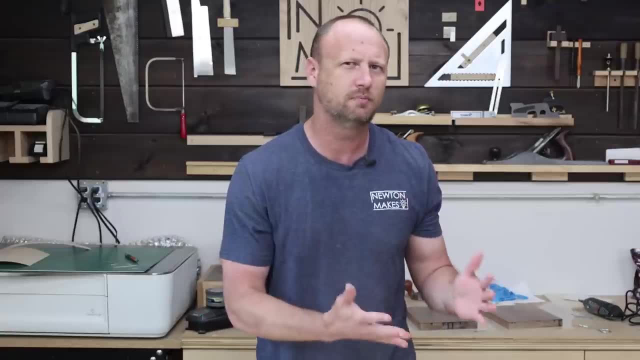 because of time and materials. But what I can compete with is the uniqueness of the item. I can provide a live edge item, a once in a lifetime type of item, a once in a lifetime type of board to a customer that those types of companies can't provide. 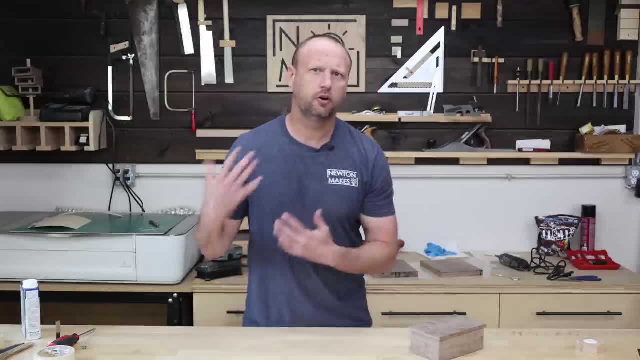 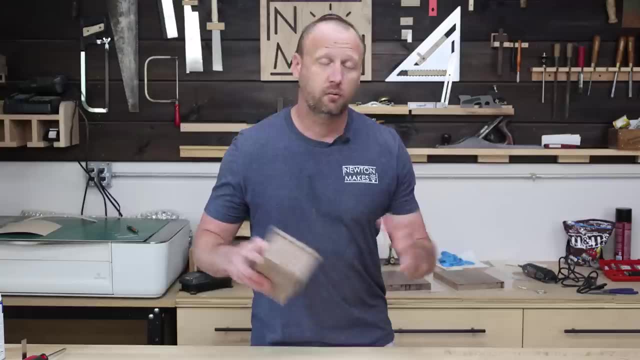 Because I focused heavily on getting these types of boards, I was able to get reoccurring customers, like restaurants that wanted more and more and more of these rare items that they just couldn't get anywhere else. Now, whether you're gonna sell boxes or candle holders, 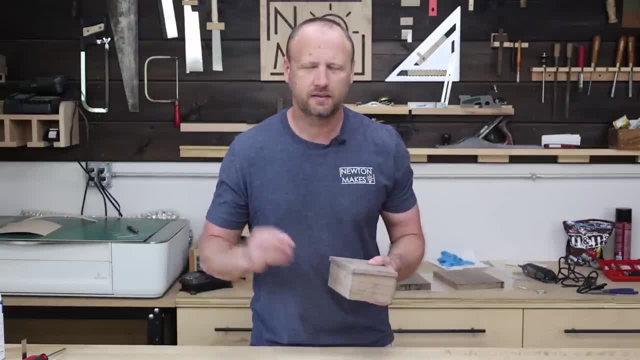 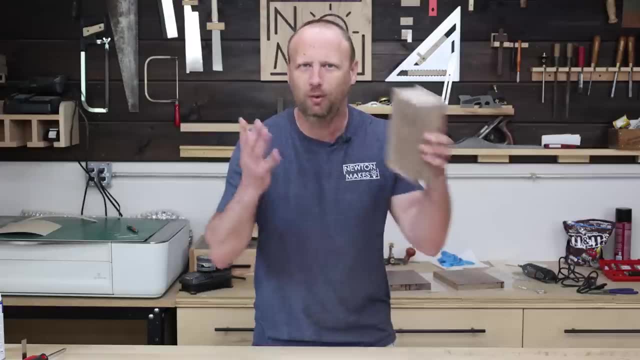 or serving boards or cutting boards or whatever else. pick a finishing method that is really simple, really easy to apply and doesn't take forever. So don't pick a finishing method that's gonna take you a whole week to get through, because you just don't have time for all that. 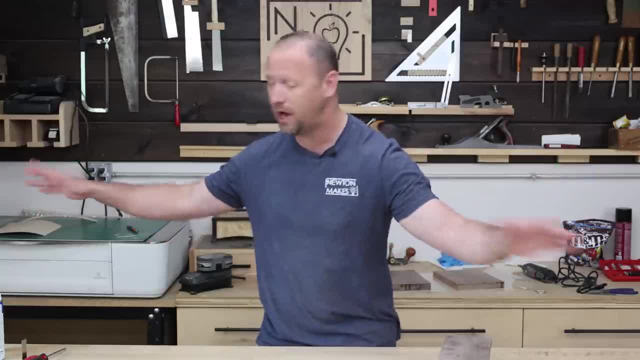 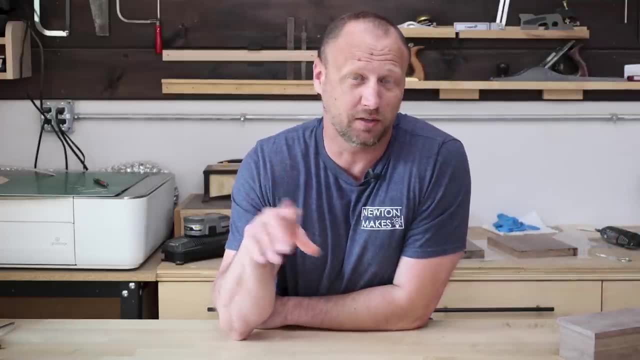 And also you probably don't have space. You're gonna make a whole lot of items You're gonna have to spread all over your shop and you ain't gonna have no place to work. A lot of people signed off after seeing the third project. 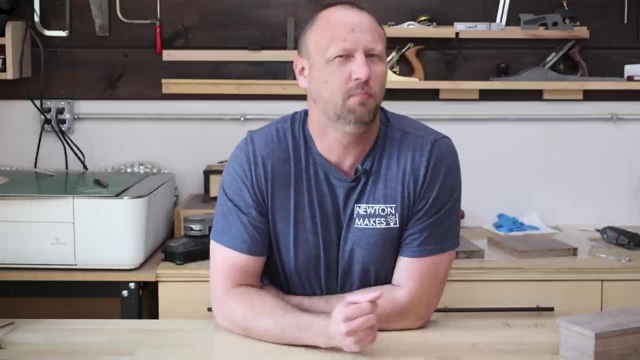 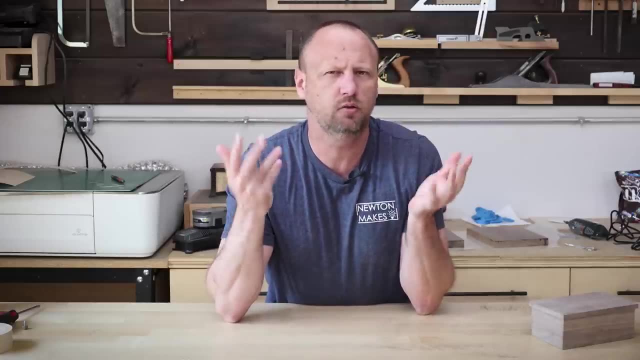 because this video talks about three different projects that you can sell, But for y'all that stuck around, I'll give you a fourth one. This bonus project idea is what completely changed my outlook on how to make money off of woodworking, And that is stop looking for regular customers. 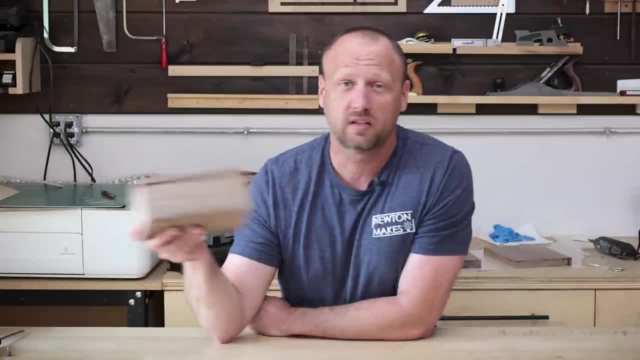 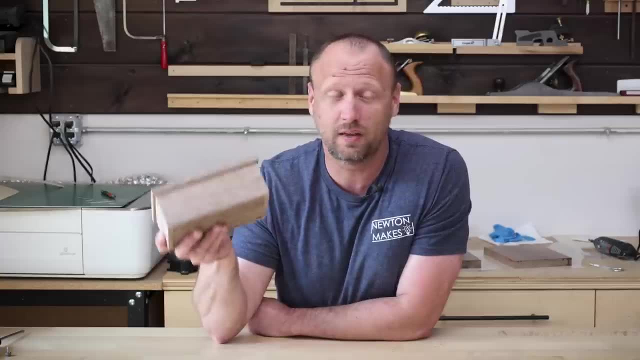 and instead stop catering to your fellow woodworkers. Let's say, I make this box and I turn around and sell it. Then I gotta make another one and I sell that, And I keep doing that until finally I just lose my mind for making the same thing. 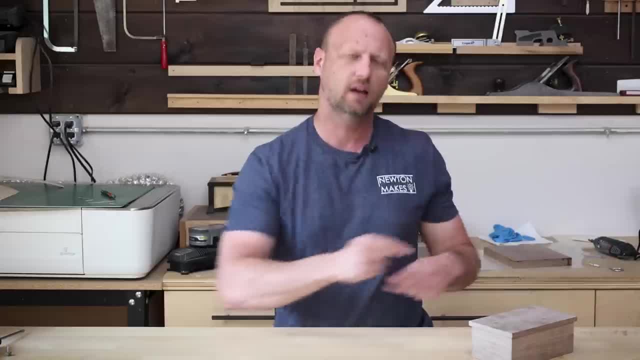 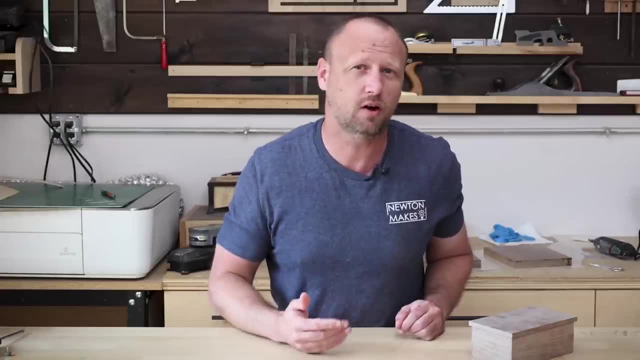 over and over again, unless that's something that you enjoy doing Now instead, imagine making that box and then selling it to an infinite number of customers, and you never have to make it again. Well, that's what I talk about when I say: